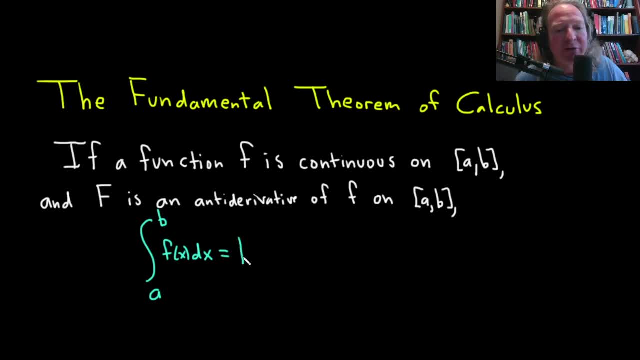 formula: This is equal to the antiderivative of little f, so big F evaluated at the uppermost limit of integration, minus the antiderivative of little f, which is equal to the antiderivative of little f, so big F, evaluated at the lower limit of integration. So it's a really cool equation. 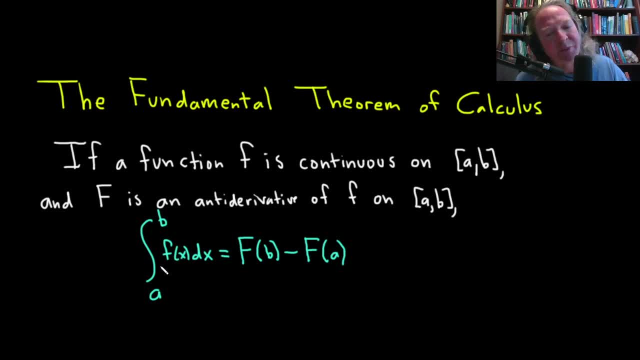 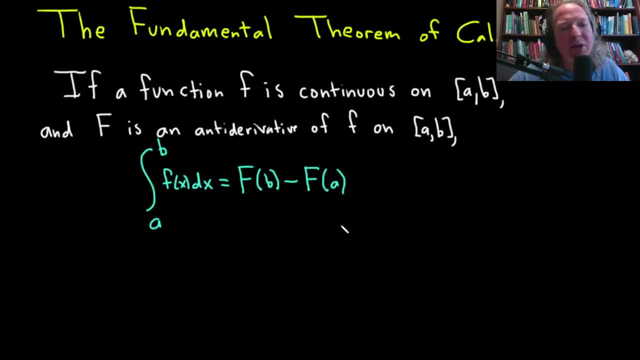 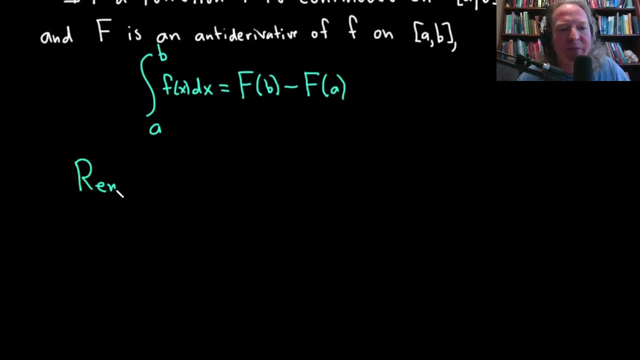 because it relates everything we were doing with definite integrals back to antiderivatives, right? So it's big, big step and it makes the computations so much easier, right, So much easier. A couple remarks that need to be mentioned here, So perhaps you know. 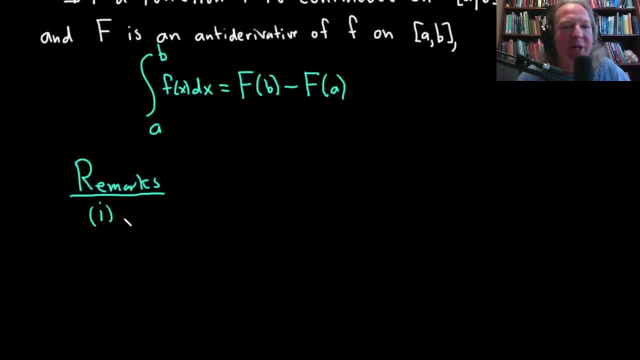 the most important remark, or an important remark, is that you don't need to write the constant of integration anymore. So whenever you're doing definite integrals, you don't need the constant of integration. So don't need, don't need to add c And two. the second: 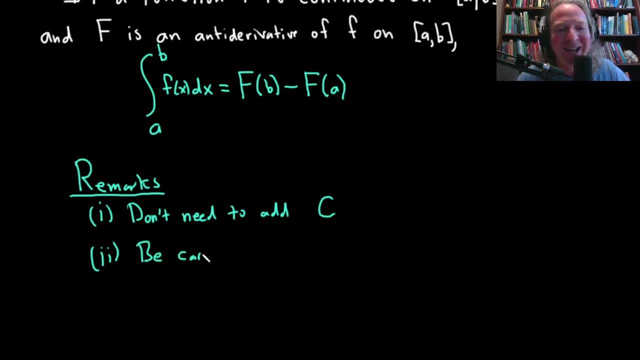 remark is to be careful. So we're working. we're going to be working with numbers now We'll have a lot of fractions, so you want to just take your time and, you know, go through things slowly. Let's start. 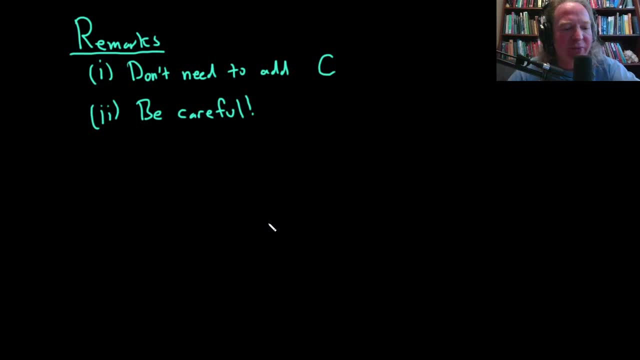 with a simple example that we can work out. So you see how to use the fundamental theorem of calculus. So let's start off simple. Let's say: we're integrating from 1 to 2, and we just have x with respect to x, So x, dx. 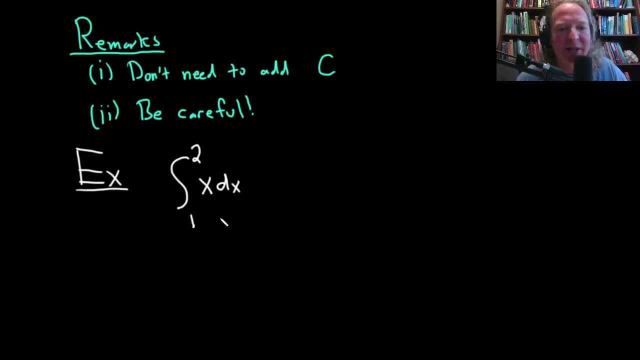 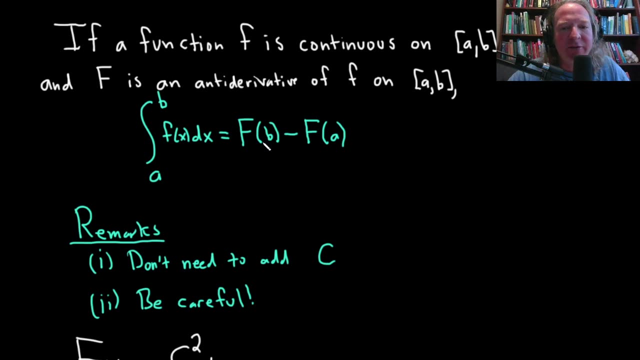 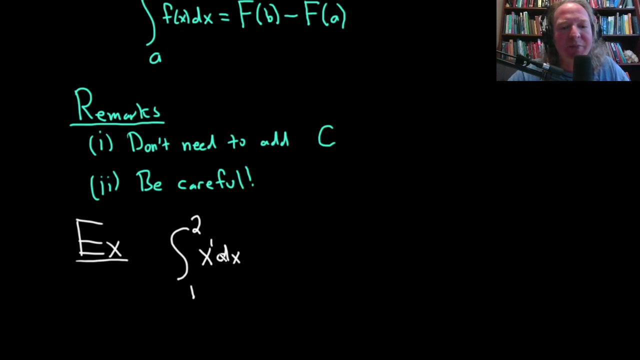 We're integrating x with respect to x. So basically, according to the formula, it's going to be big F of b minus big F of a. So typically what you do is you just integrate it and then you don't write the c. So here we'll use the power rule. So you add 1 to 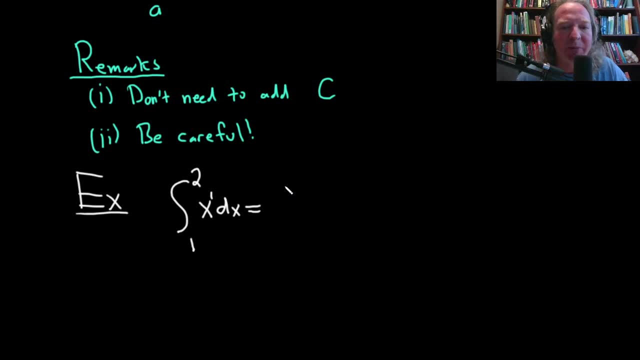 the exponent. so it's x squared, and then you divide by 2.. So it'll be x squared over 2.. Normally you'd put a plus c, but you don't have to put a plus c Just to indicate that. 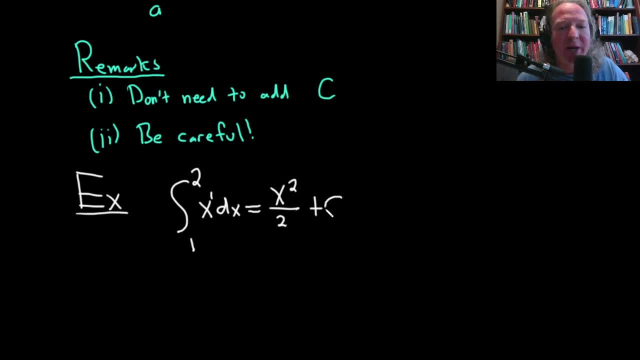 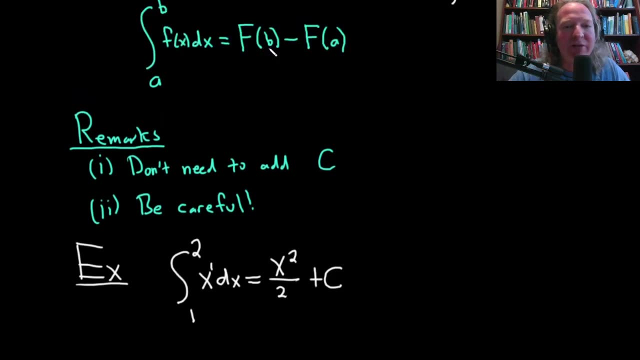 you don't have to. I'm going to put it this time, just so you see what happens. So this is just the antiderivative right. This is wrong. We have to have the antiderivative evaluated at the top limit of integration, the upper limit, and then subtract it from. 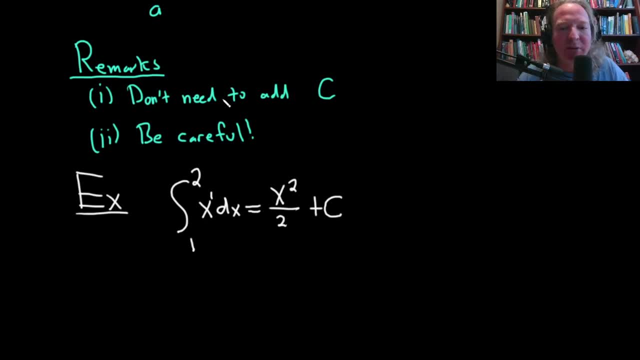 the antiderivative evaluated at the lower limit. So what I'm going to do is I'm going to use a double bracket like this, and I'm going to put a 1 here, I'm going to put a 2 here, And what this notation tells you is that you first plug. 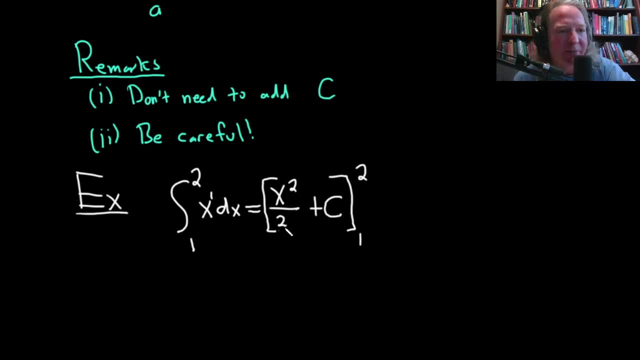 in the 2, right, Because this is your big F of x, right here. Let me just circle it. This is big F of x. So if you plug in a 2, you get 2 squared over 2 plus c. That's big. 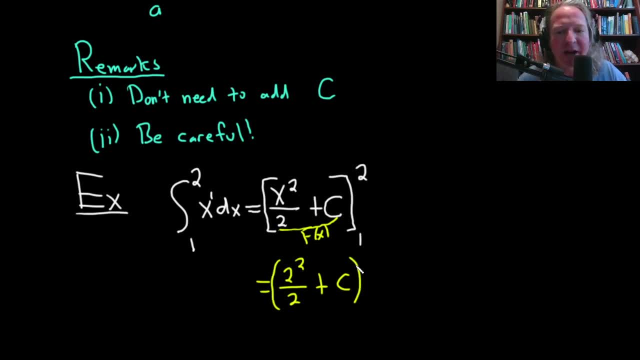 F of 2, right, Because you plugged in 2 into big F minus and then plugging in 1 to big F, it's big F of 1.. Let me see that, So let me just scroll down here and write it for you. So this is big. 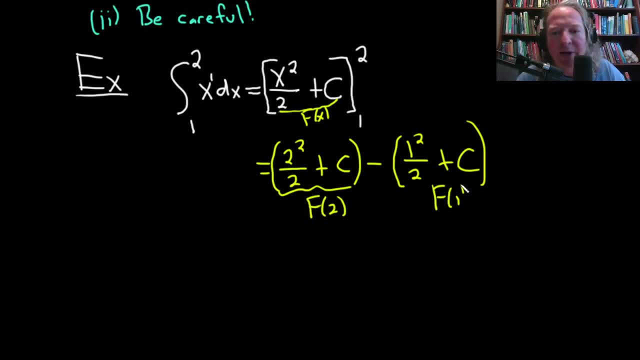 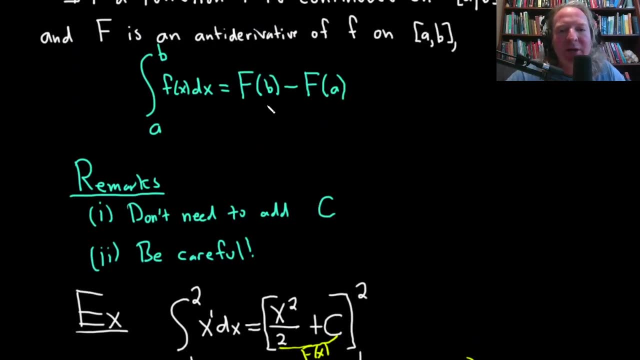 F of 2, and this is big F of 1, right, Just using the formula, which again is F of b minus F of a. I think a lot of people don't actually think about the formula, which is fine, You. 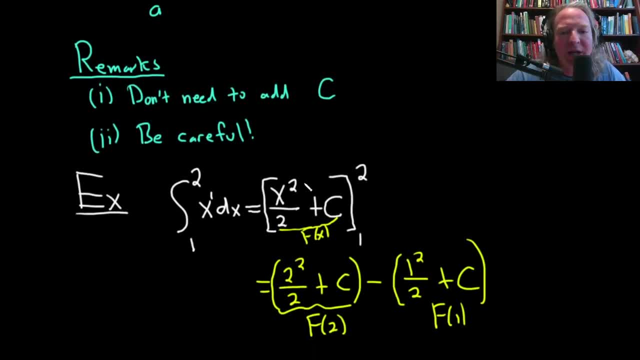